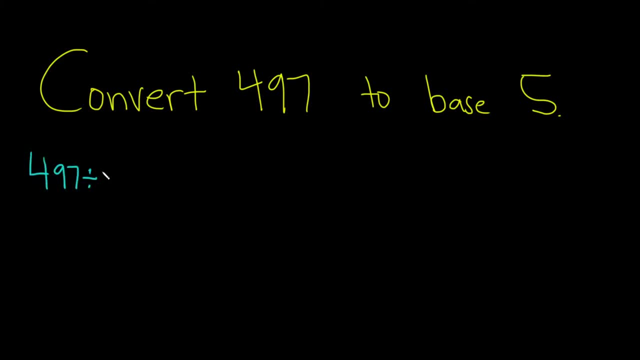 497 and you divide it by 5. And we care about the remainder. Okay, so if you just use a calculator and you type it in, you get 99.4.. So that means that 5 goes into 497 99 times. So if you do 99 times 5 and you put that in your 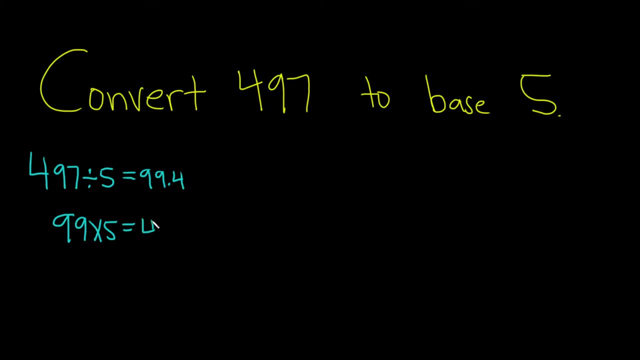 calculator, you see it's 495.. So now you can find the remainder. You see, so 5 goes into 497 99 times. And what's left over? Well, you just subtract these numbers: 497 minus 495.. So 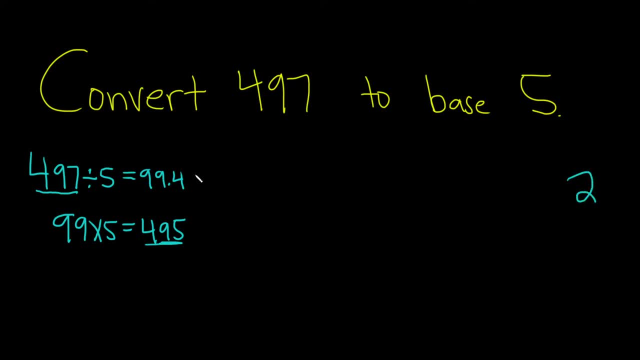 the remainder is 2.. So I'm going to write it, I'm going to write it over 2.. Then you do it again, but you do it with this number here. So 99 divided by 5.. So if you put: 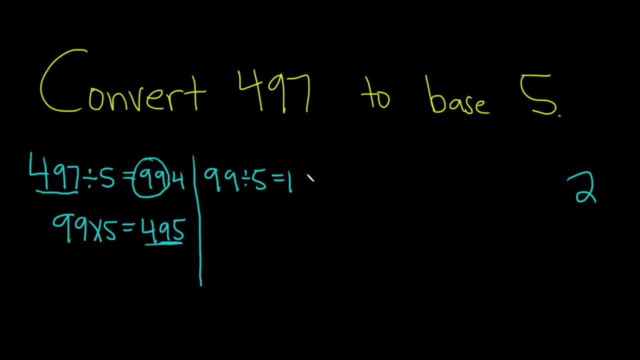 this in your calculator, you get 19.8.. So again, we're looking for the remainder. This means that 5 goes into 99, evenly 19 times. There's the fractional part left over. We want to figure out what that is. So what you do is you do 19 times 5 in your calculator, Just all calculator. 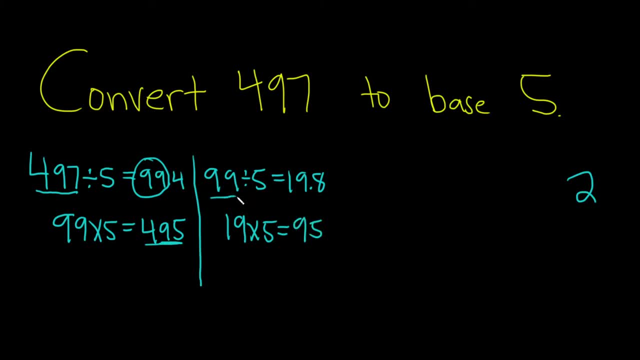 work. This is 95. Then you subtract, So you get 4.. So the remainder is 4.. Then you do it again And again. you take this number 19 divided by 5.. So this should be like 3 point something. Let's see. 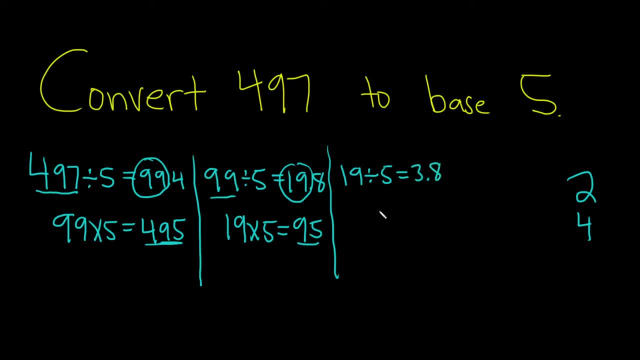 Yep 3.8.. So 3 times 5. You take this number, multiply it by 5, you get 15.. Then you subtract, So you get 4.. The remainder is 4.. Then you do it again. 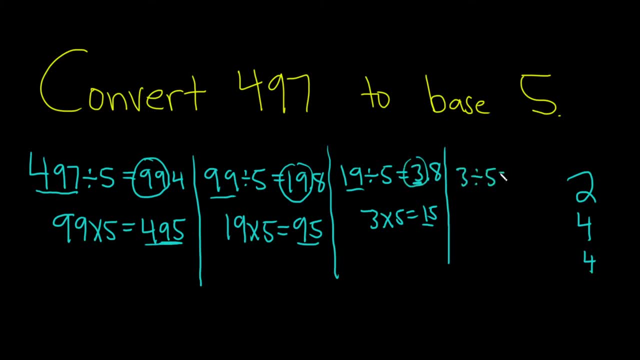 take this number and divide it by 5.. 3 divided by 5.. Now, this is going to give you 0.6 in the calculator. okay, So what's the remainder? Well, in this case, the remainder is just 3,. 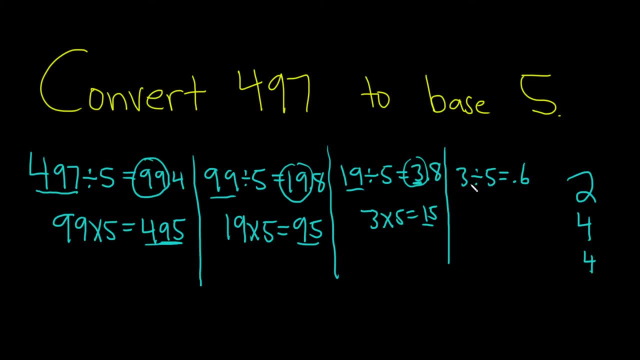 okay, Because 5 goes into 3 zero times and the remainder is 3.. So 3, right, It doesn't go in at all. So the whole thing is the remainder right. And now what you do is you just read: